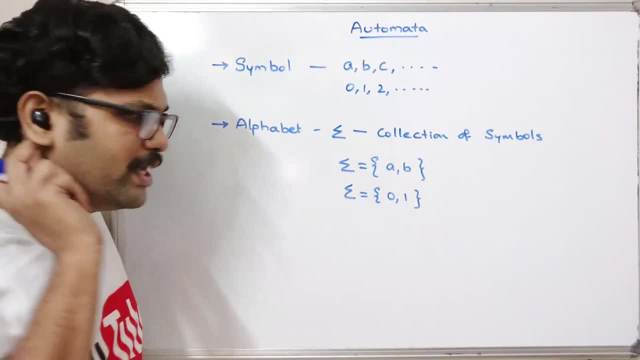 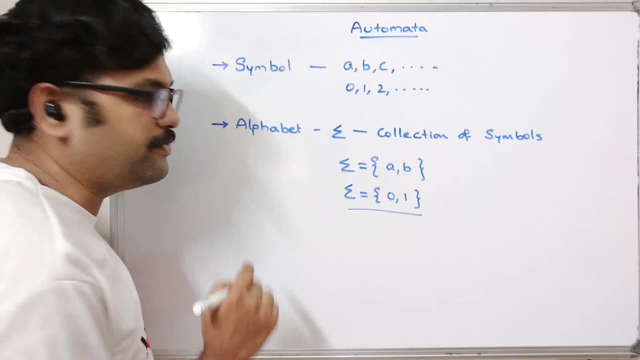 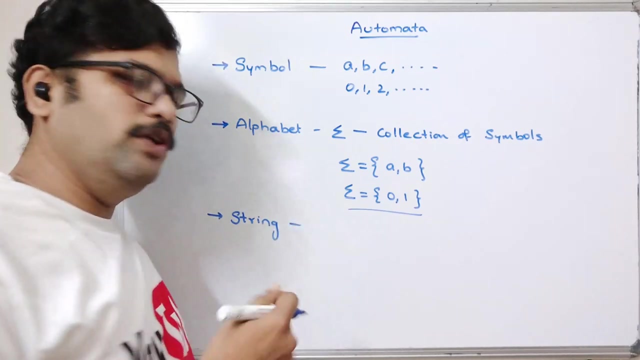 So this is another alphabet, binary alphabet. We can simply call it as a binary alphabet. So this is the alphabet. It is a collection of symbols, A collection of symbols, And the next one is string String. So generally we know that a string is a group of characters. 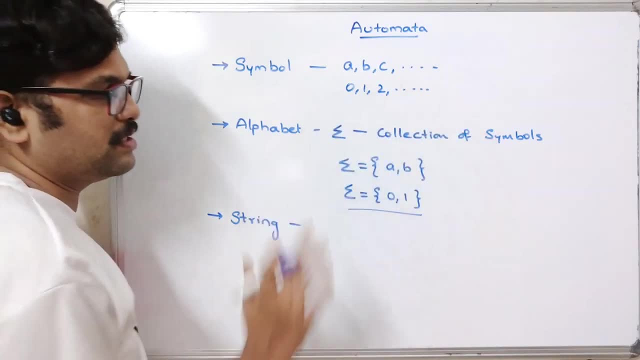 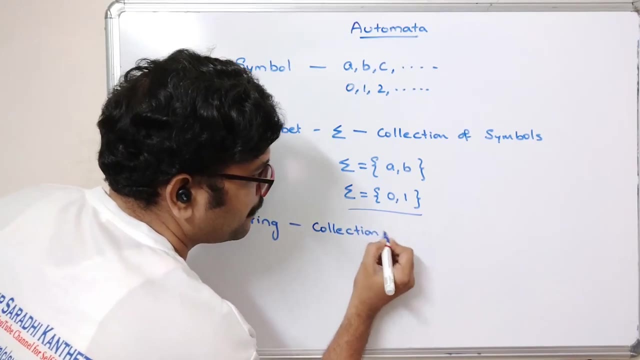 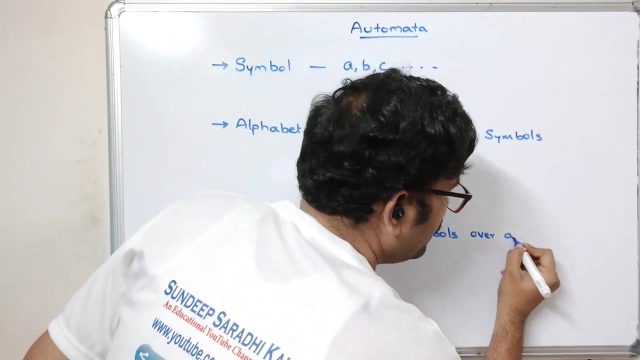 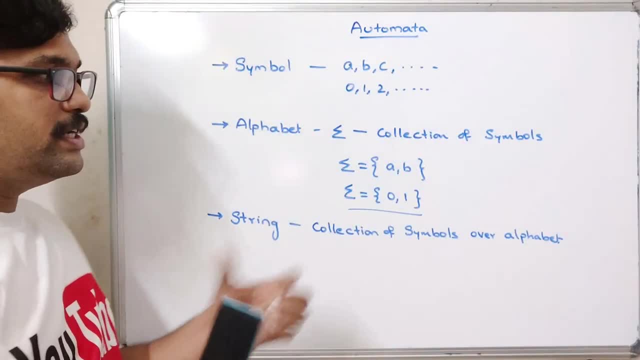 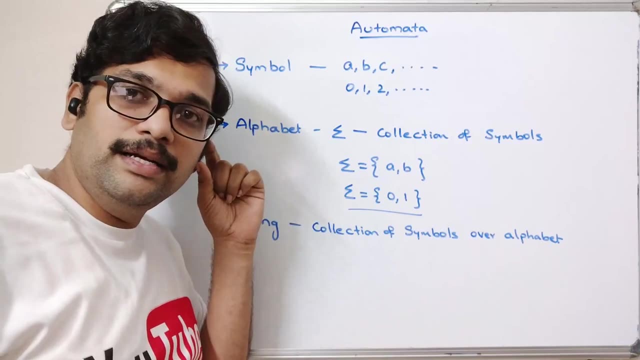 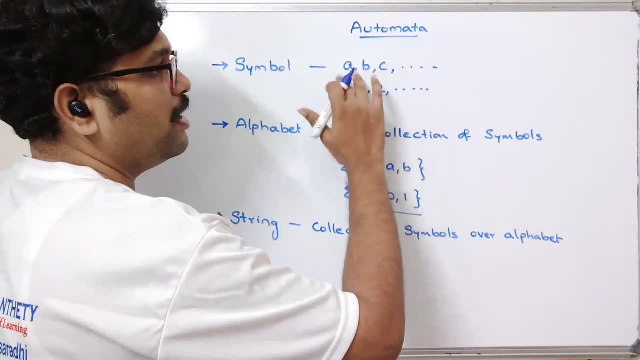 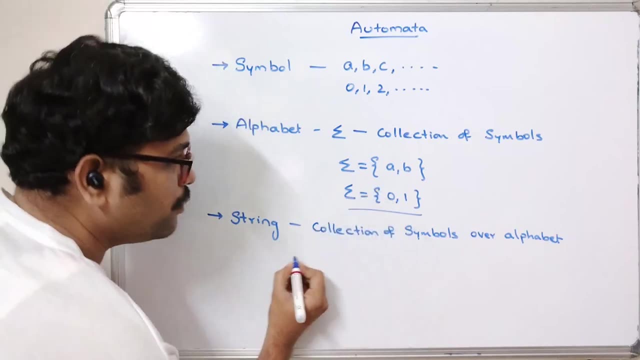 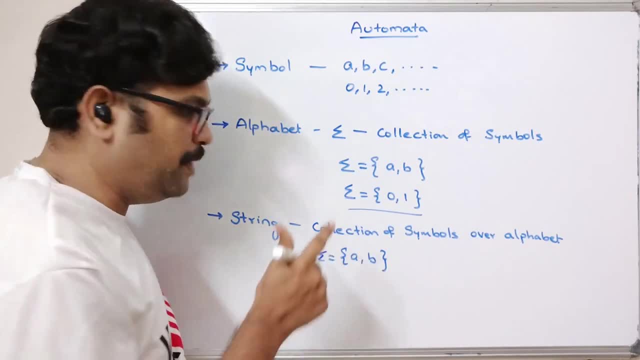 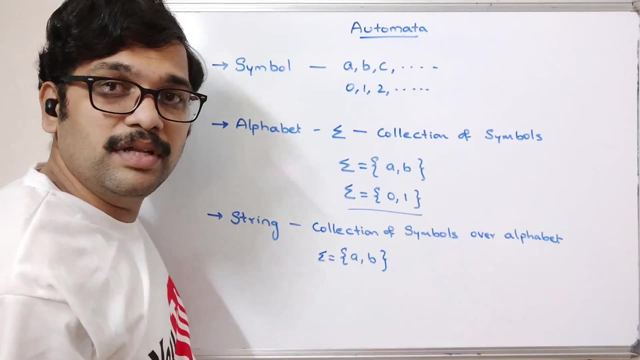 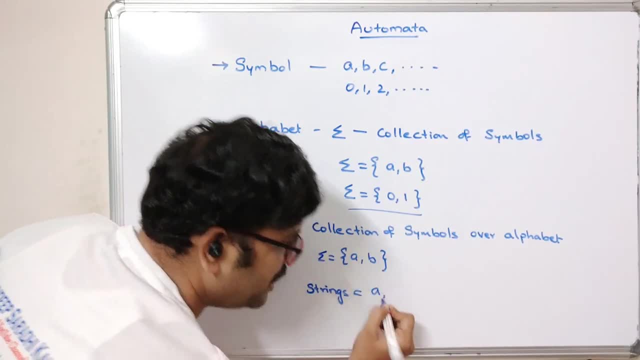 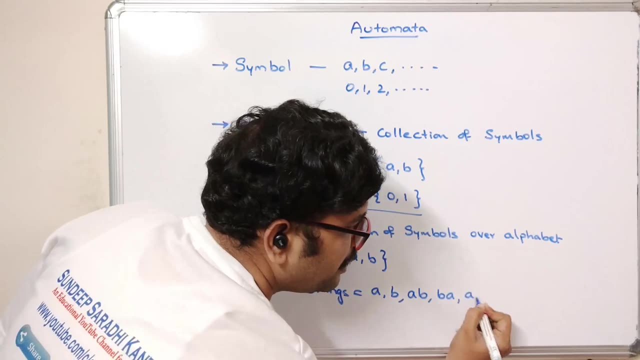 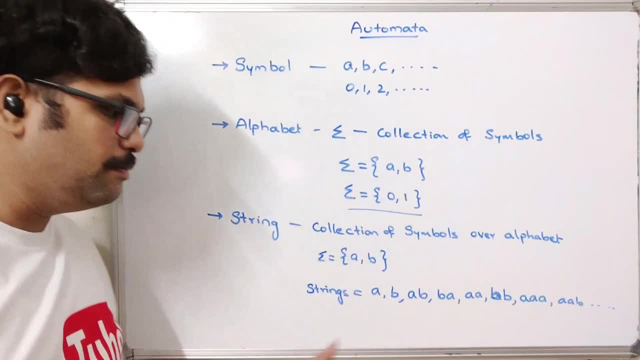 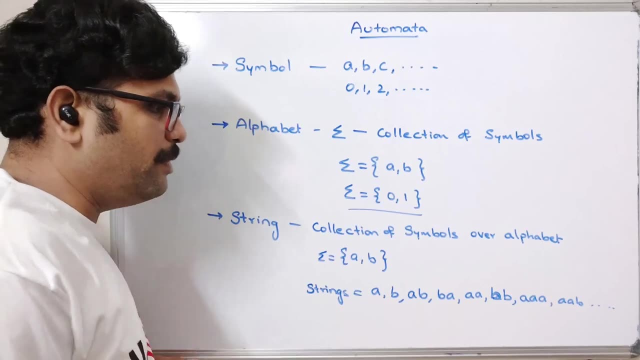 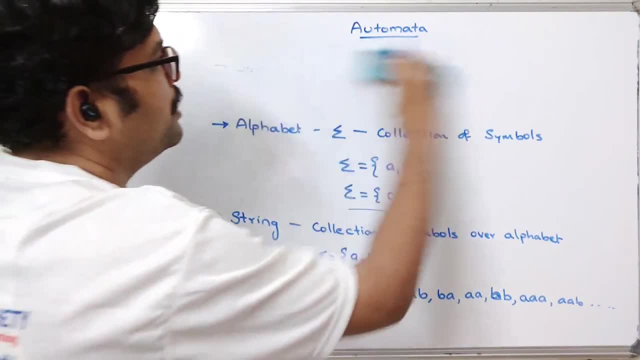 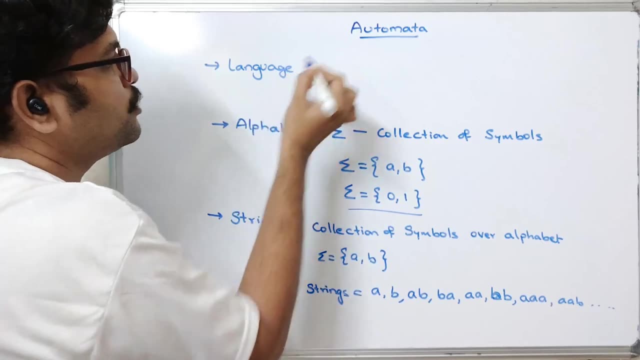 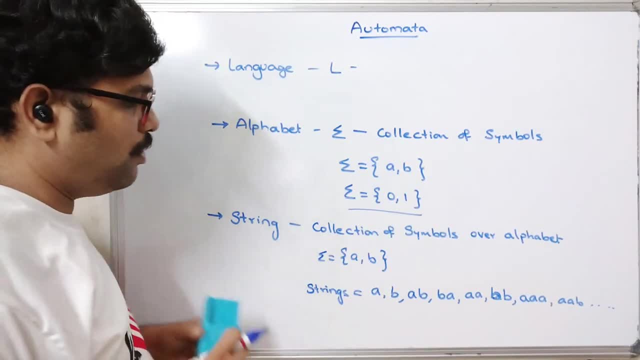 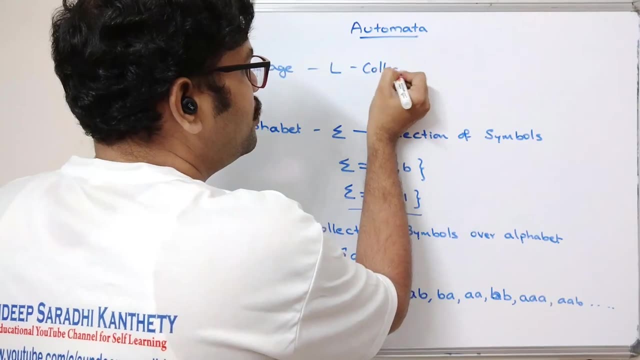 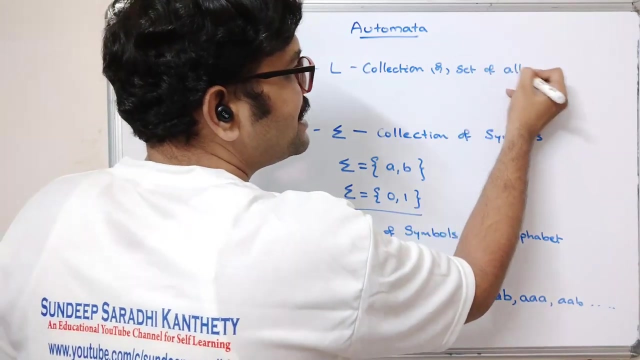 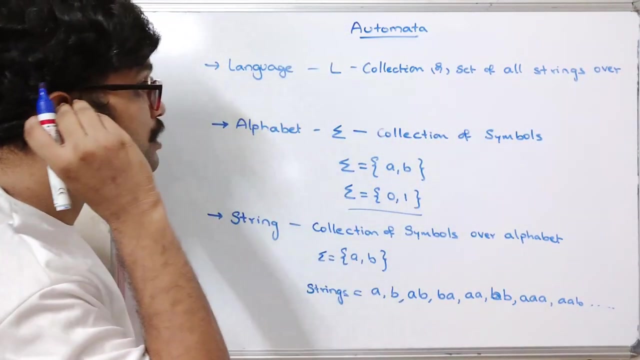 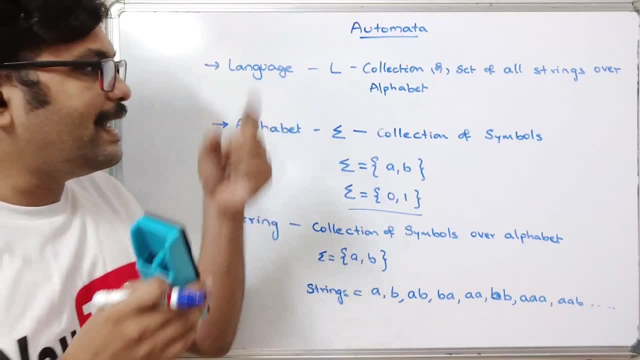 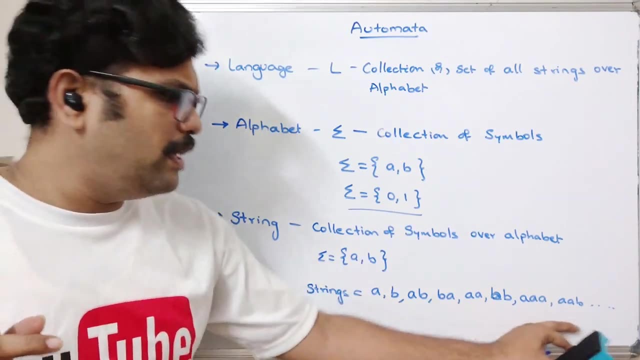 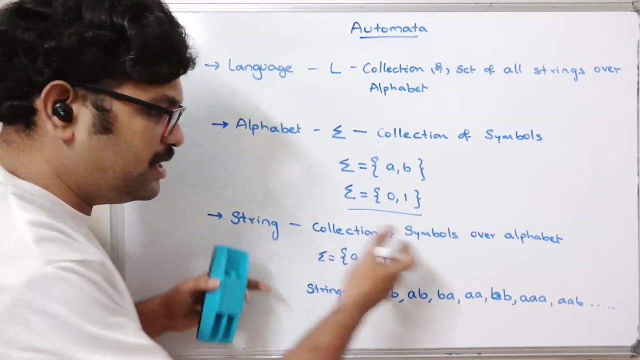 is called language, so that language can be having set of all possible strings. so here we can have a multiple number of strings. we can have a multiple number of strings. that is the infinite, because here there is no specified length, right? so this is infinite length. so all these strings, 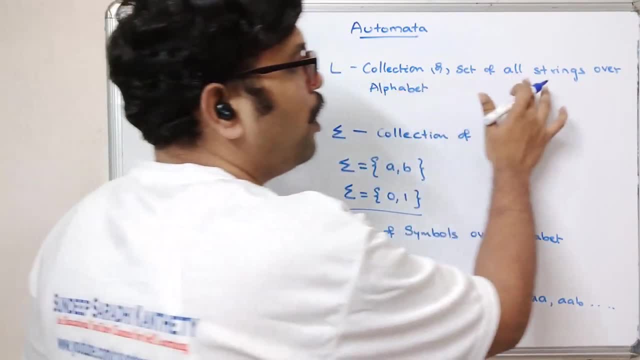 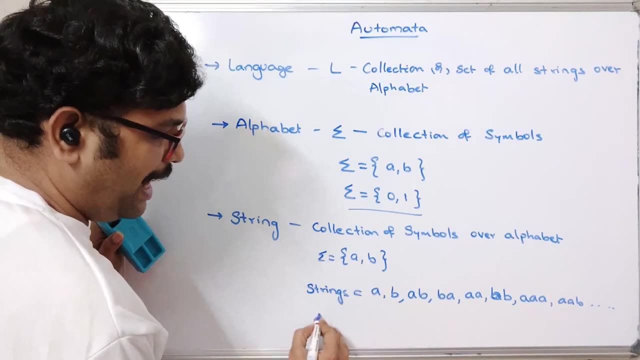 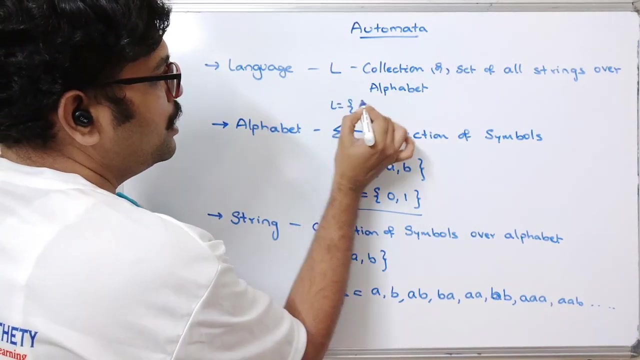 combinedly known as L, so a set of all strings over the alphabet right now. so, if you consider this example, so L is equal to. it is nothing but a set of all the strings. so L is equal to. so we can use A, B, A, B A A. 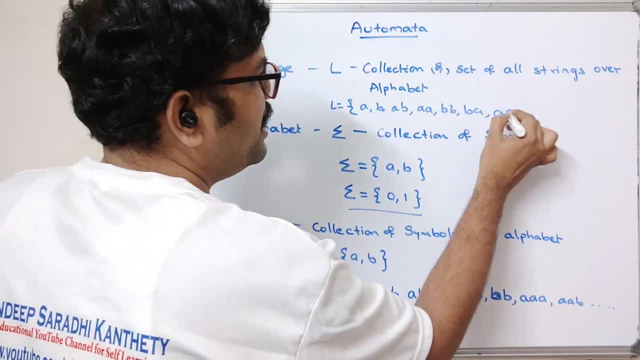 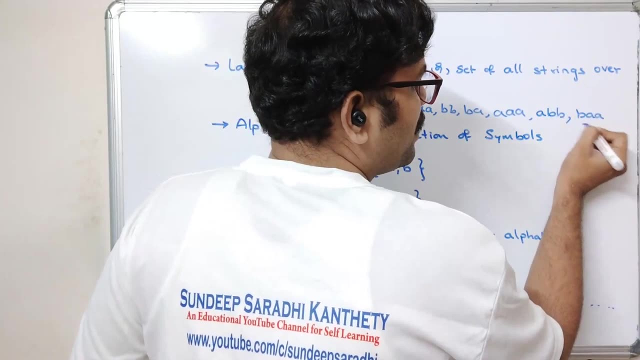 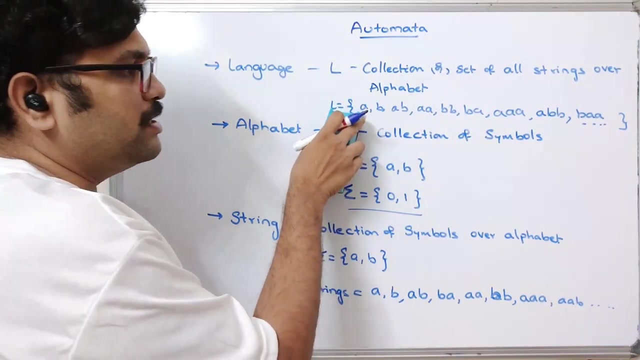 and so all these set of all strings, so we can use a, B, A, B A A and bb, ba and a three digit, three symbols, okay, length, length, three. okay, so abb, ba, etc. so after the three length we'll go with the four length, right? so this is called a language. language is a set of. 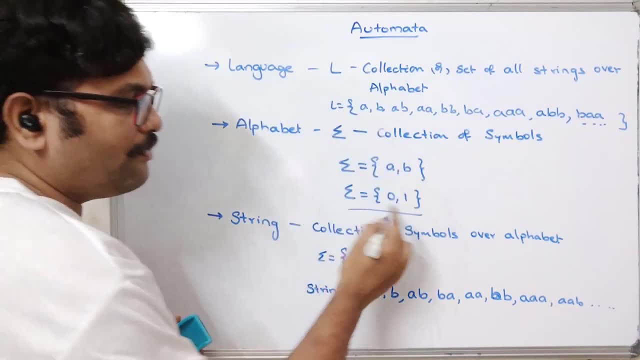 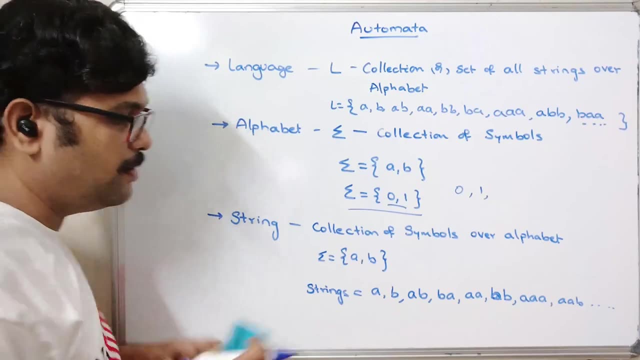 all strings over the given alphabet. so if the alphabet is 0- 1, we'll be having the combination of all the zeros and ones. the strings will be having the combination of zeros and ones. okay, now hope you understood about these things. so what is meant by? 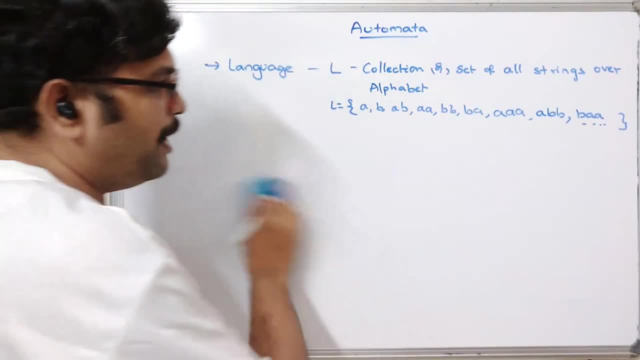 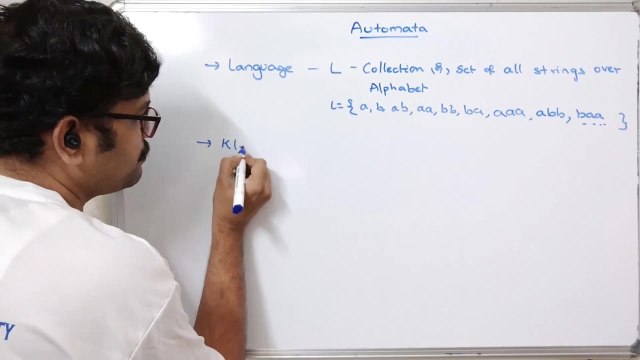 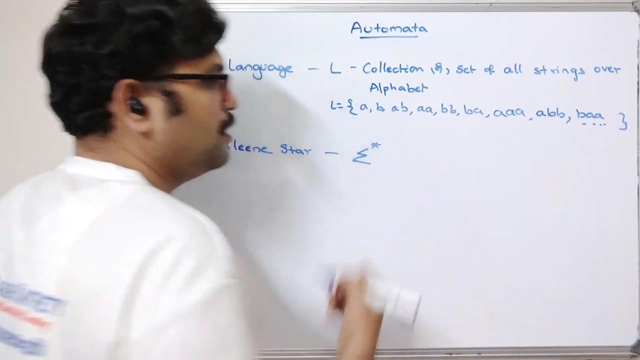 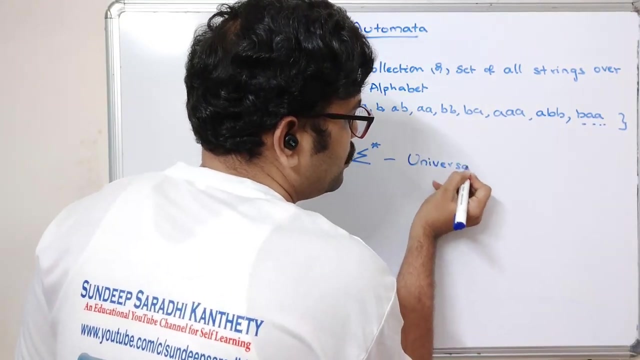 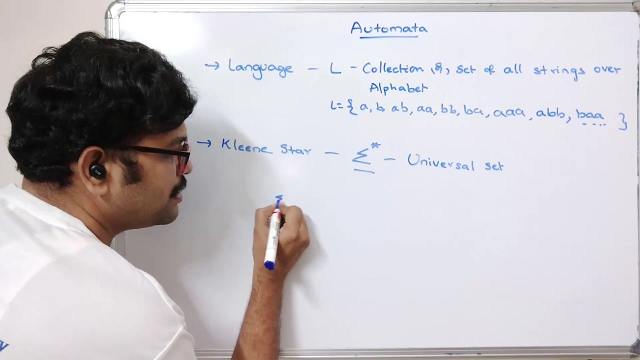 the symbol, alphabet, string and the language. now the next one is clean star, clean star. so clean star is usually represented as sigma star, sigma star so, which is also called as universal set, universal set or universal language, universal language. so this sigma star is nothing but sigma star is equal to. it can be calculated as sigma 0. 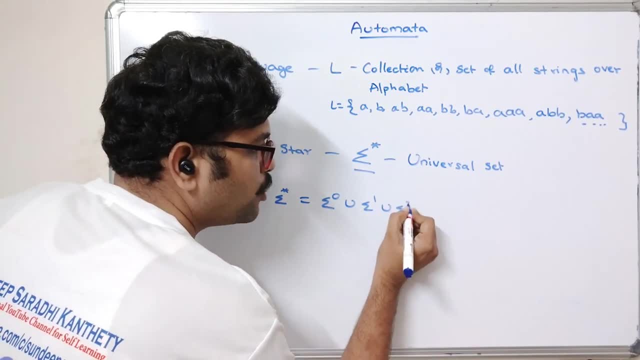 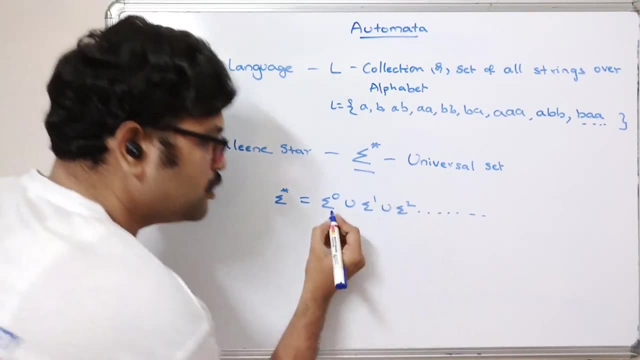 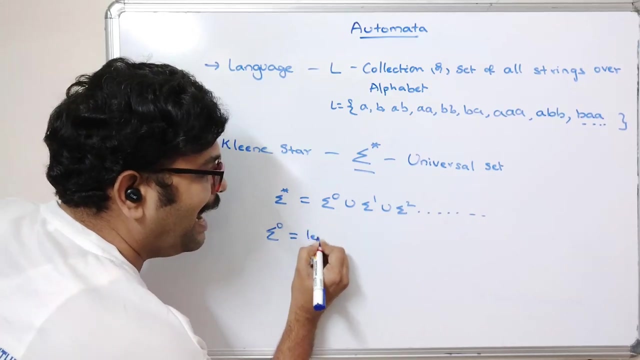 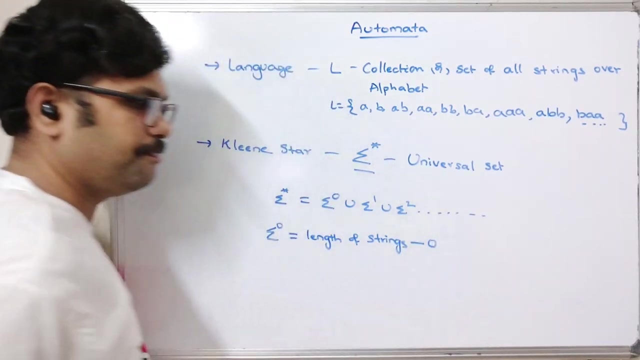 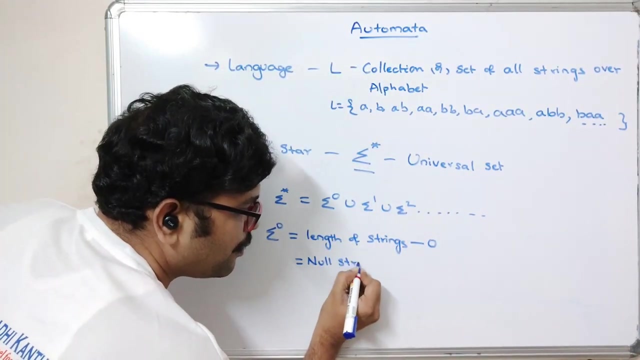 union sigma 1, union sigma 2 and so on. okay, sigma star is equal to sigma, not union sigma 1. so where this sigma 0? sorry, sigma 0. sigma 0 means length of strings. length of strings must be 0, length of strings must be 0 and this will usually called as null string. null string or empty string. 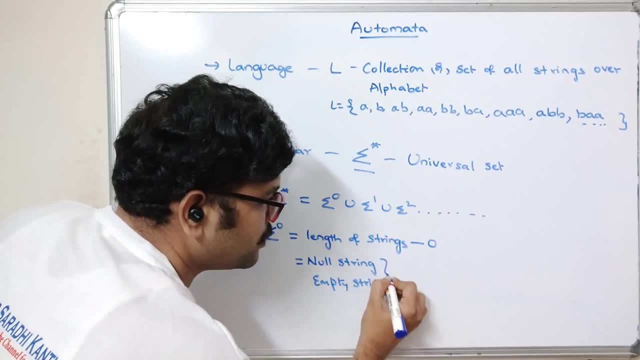 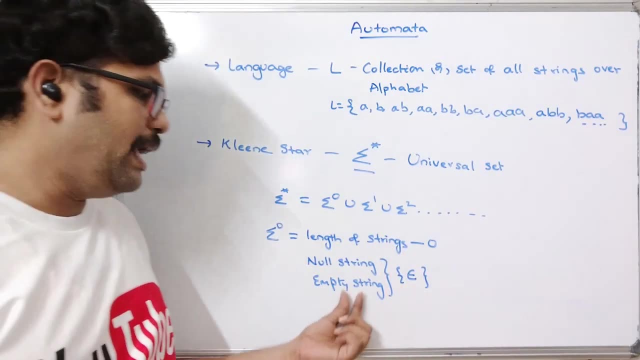 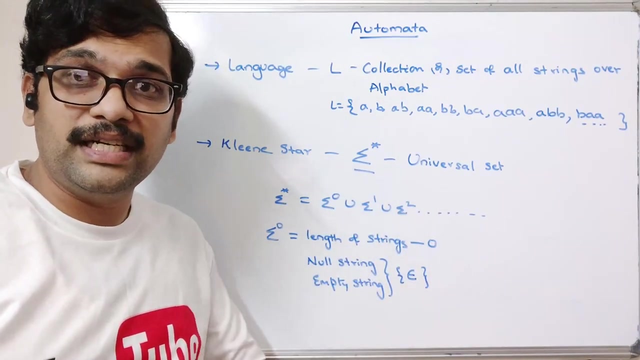 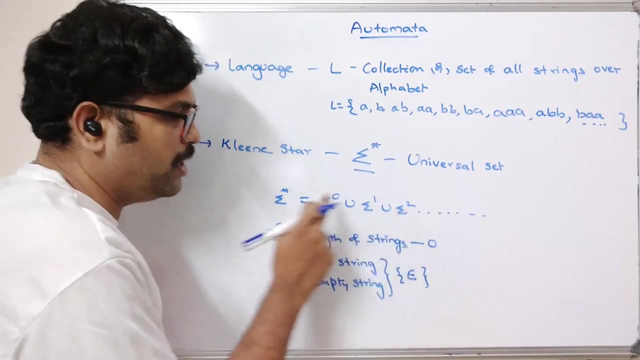 okay, null string or empty string. so this- a null or empty string- is represented as null string or empty string is represented as epsilon. so here epsilon means length of string is 0, length of string is 0, so this is also included in clean star. that means sigma star. this should be also be included in clean star and similarly hope. 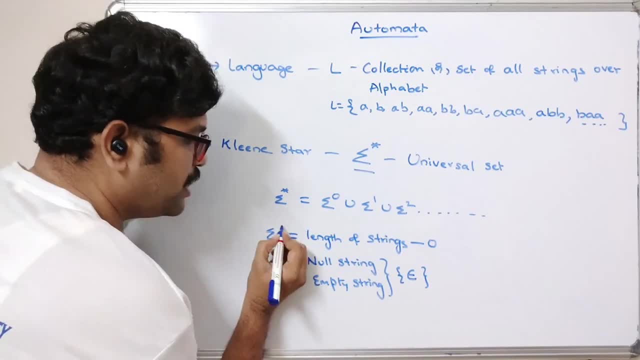 you understood this sigma 0. now we'll go with the sigma 1. so if you consider sigma 1, if you consider sigma 1, the length of the strings must be 1. the length of the string must be 1. the length of the string must be 1. 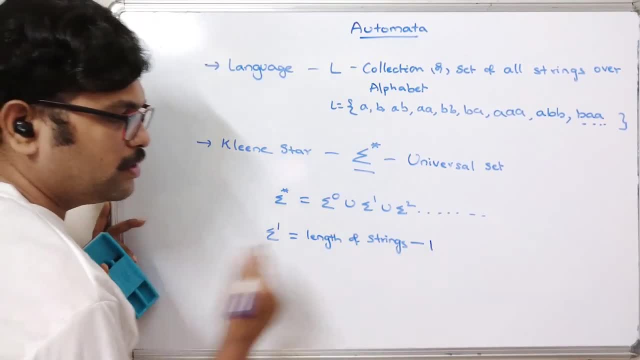 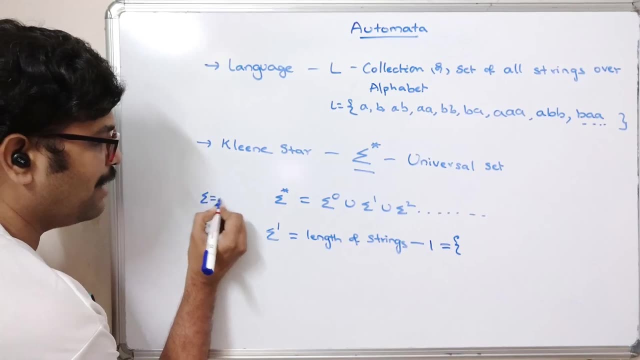 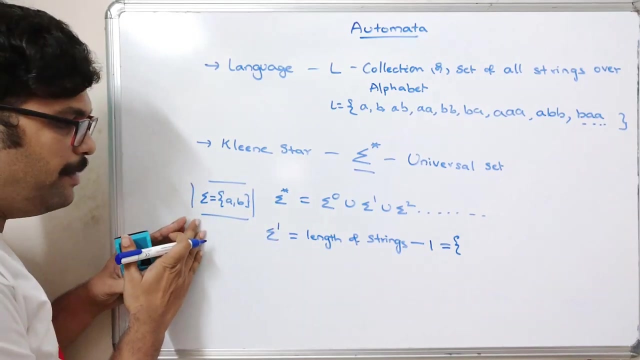 so usually the length of strings must be if the length of string is 1. so what are the possible string? for example, if you take the alphabet as bite, you take the alphabet as ugh, you from this alphabet. so consider all the strings. length is equal to 1 to string. so simply we can say: 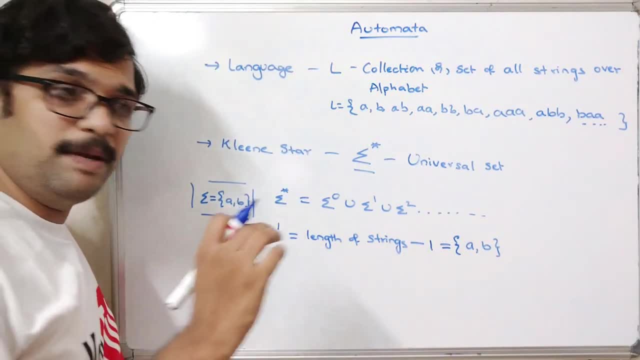 Damit. these are the strings which can be possible with this alphabet of string. now, when I am concentrating on thejerake, Aaa, copper, be, now from this alphabet. so consider or construct: all the strings with length is equal to 1, so simply we can say: acaba, be. these are strings. 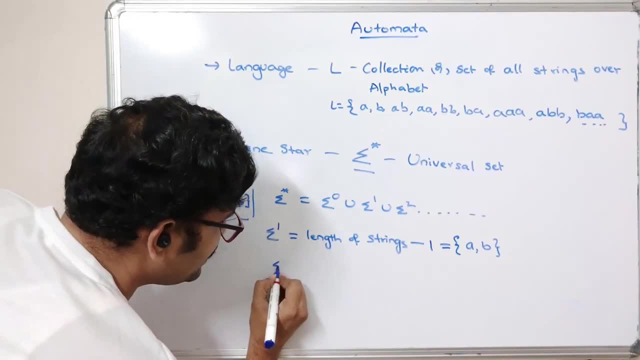 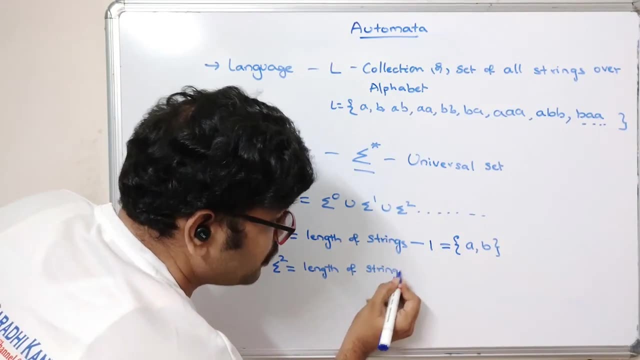 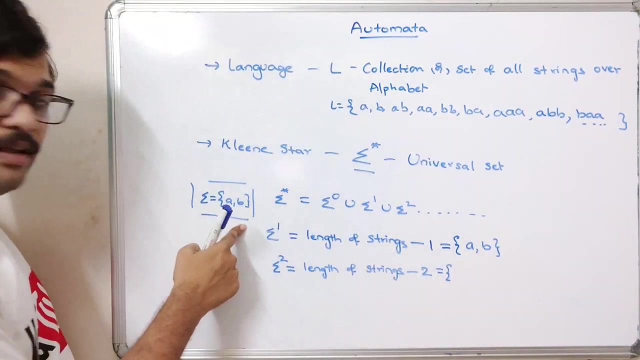 way of strength of length 1, now Sigma 2. so here the Sigma 2 means length of string strings, all the strings with 2, length of all strings with 2, so the combination of a and b of length 2, so we can simply write it as a comma: a, a, b, b, a. 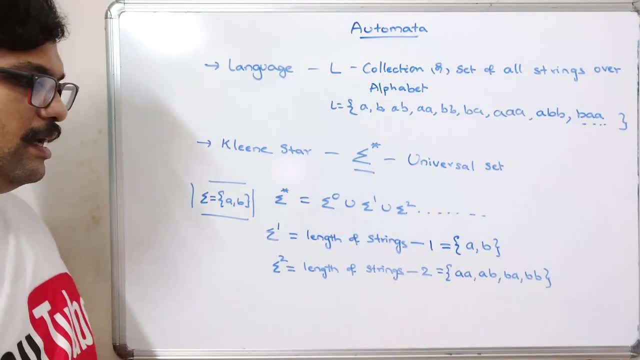 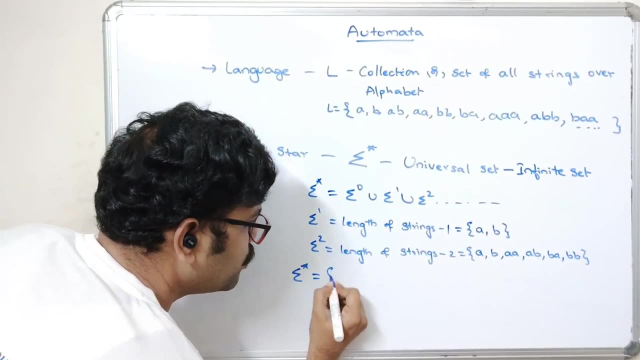 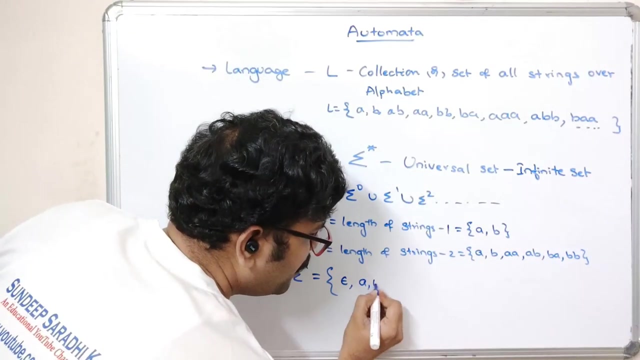 b, b. this is the length of the string now. so here you can see, the Sigma star is equal to all the strings with length 0, that means epsilon. all the strings with length 1, that is a comma. b. all the strings with length 2, so a, a. so here we. 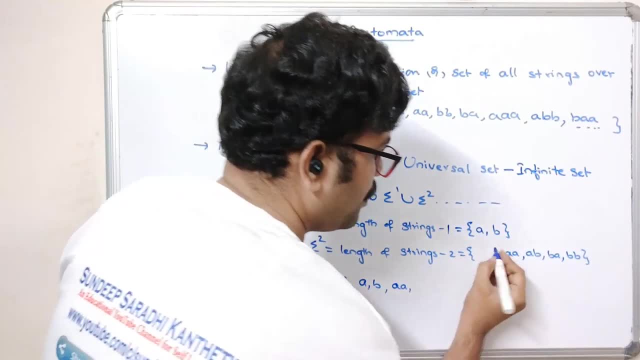 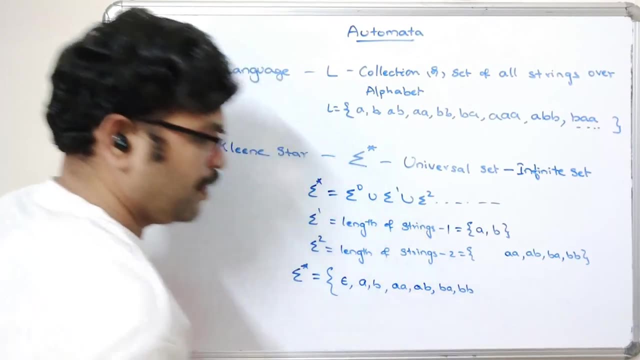 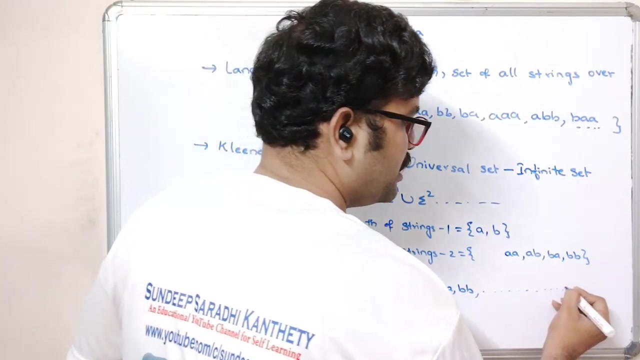 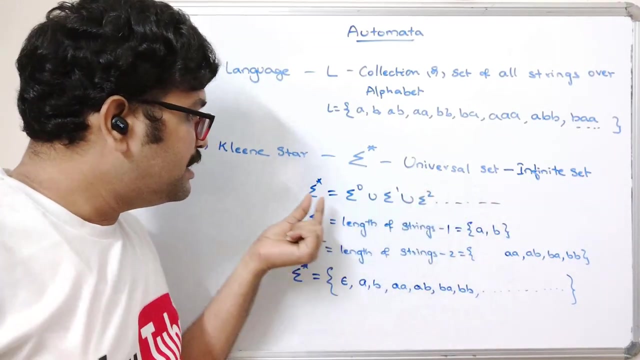 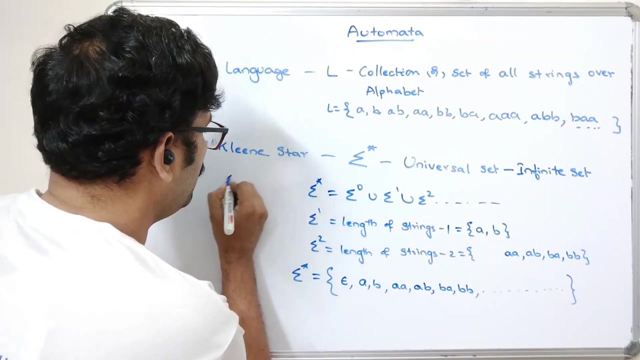 will get only a, a, a, b, b, a, b, b. so and then the length of strings 3 and so on. so you can say this one right. so that's why this is called infinite set and it's a universal set. so this clean star will be having all possible strings over the alphabet a. 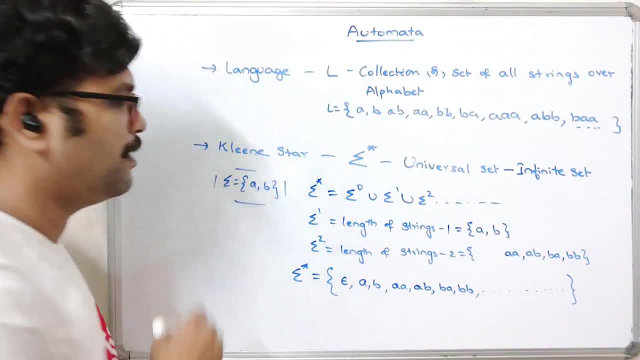 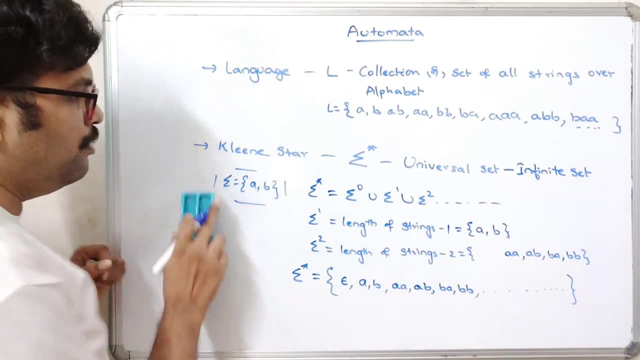 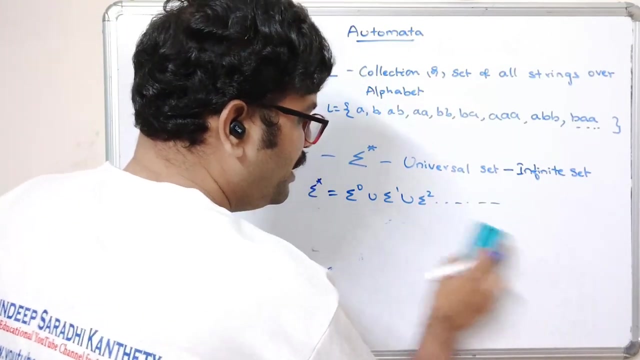 comma b right over the alphabet a comma b, so it will accept all the strings. okay, with a different lenth. now there is one more concept called, so hope you understood this- clean star right. so including the length of strings with 0, that means a墠 string, and there's one. 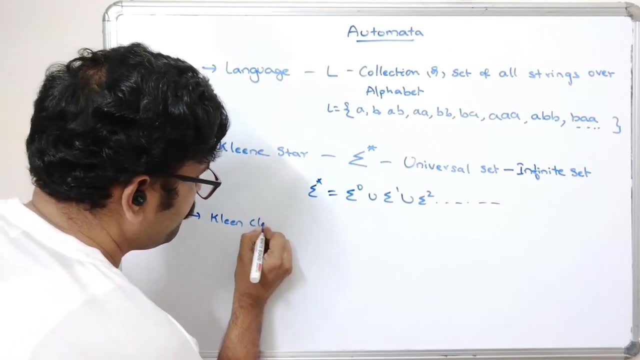 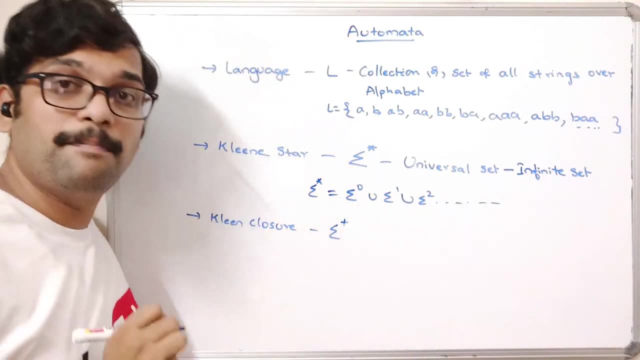 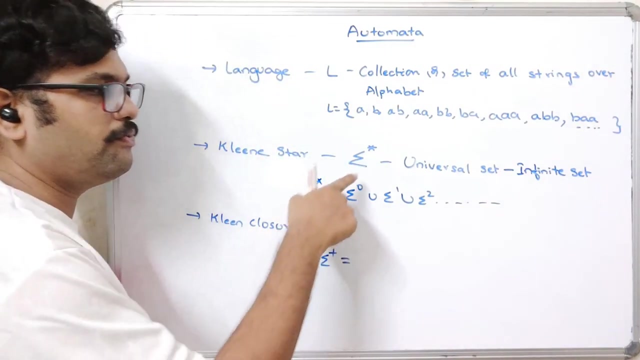 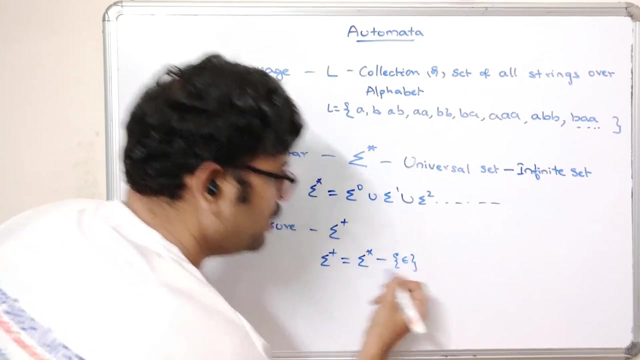 more concept called clean closure, clean closure so, which is represented as sigma plus sigma plus. so here the sigma plus can be defined as: so this is a subset of this universal set, because so sigma star minus epsilon is called a sigma plus, sigma star minus epsilon. 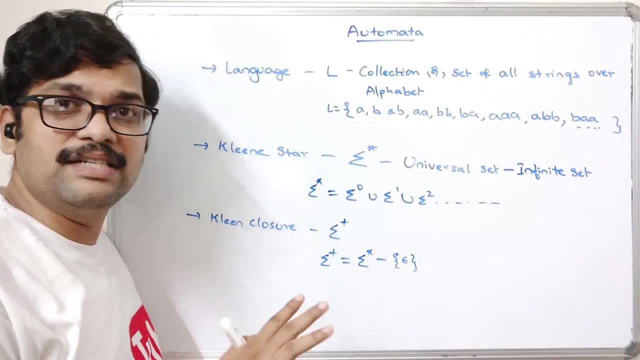 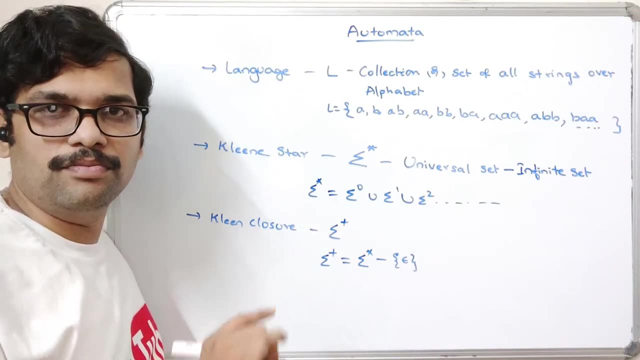 means. so it will also accept all the strings with a different lengths, but excluding the null string. so that means it should not accept the strings with length 0,. okay, this is. epsilon is nothing but a null string, so we should not include that null string inside the epsilon. 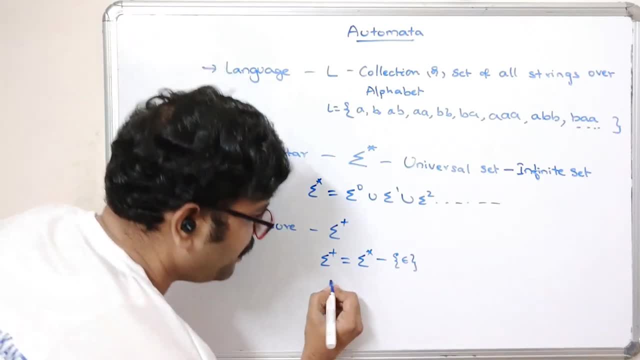 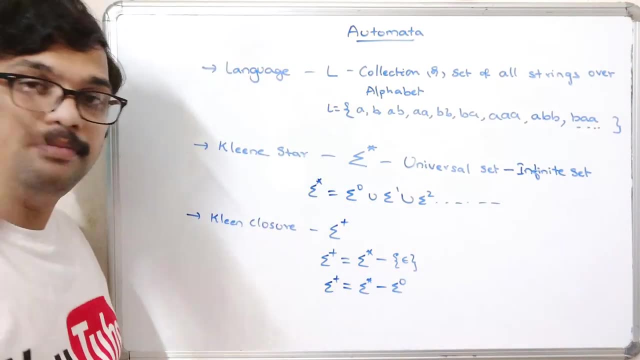 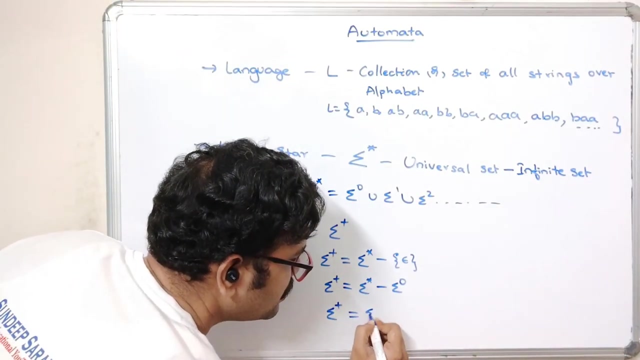 star. so that is called a clean closure. so this can be written as: sigma plus is equal to sigma star minus sigma naught, sigma star minus sigma naught. Okay, And once again we can also return this one as sigma 1, union, sigma 2, union, sigma 3 and. 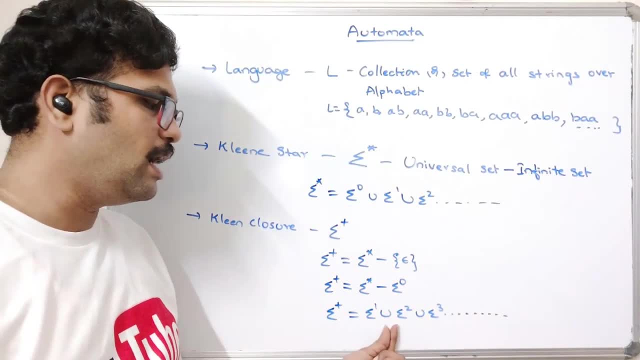 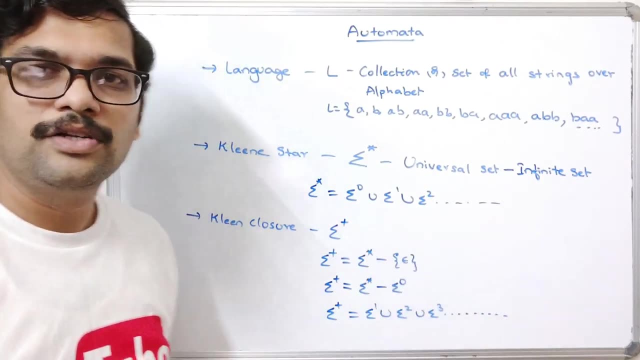 so on. okay, so what we have done? so we have started a union from 1 itself. so length 1, length 2, length 3 and so on. so this is called a clean closure, sigma plus sigma plus right. 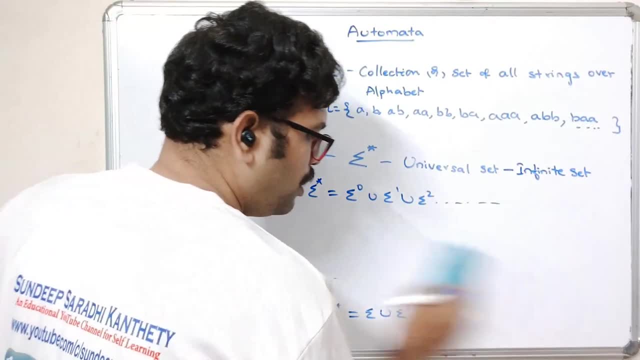 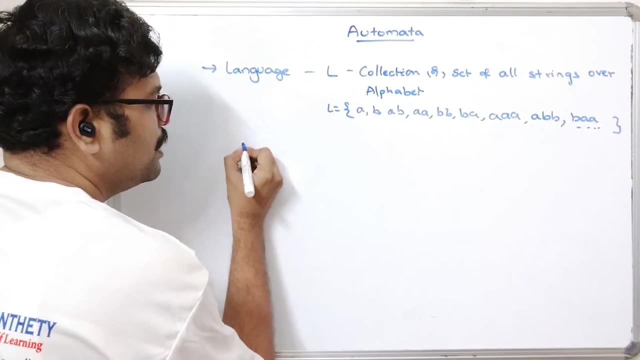 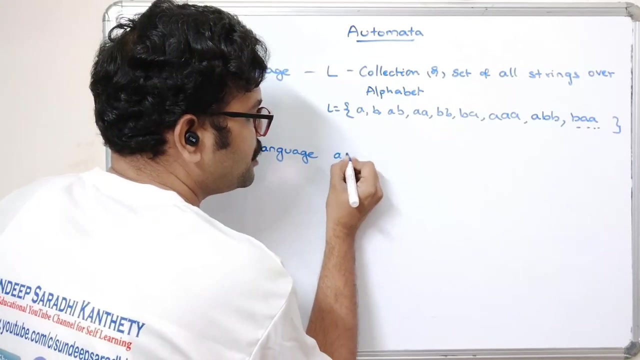 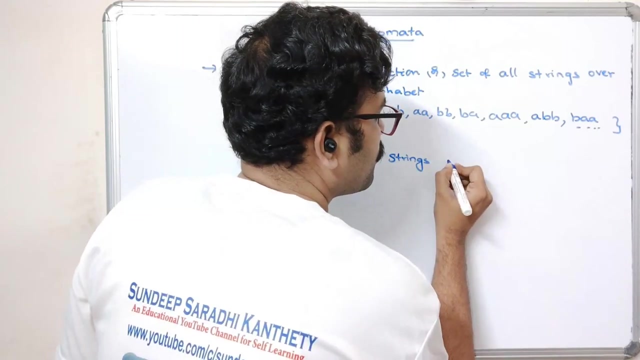 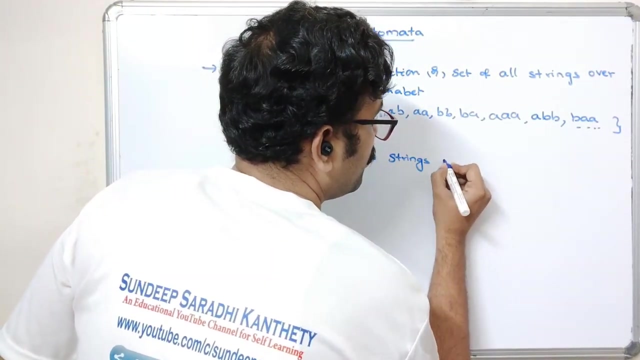 now. so the language. we will see a small example for this language. Okay, With clues. Hope you understood this. basic concepts. so, if it is so, construct a language, language which accepts strings. strings: see strings with length. 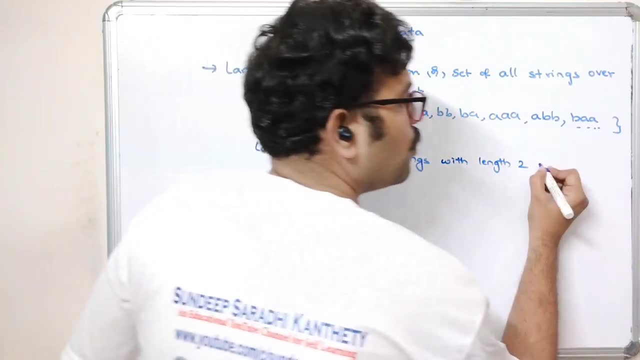 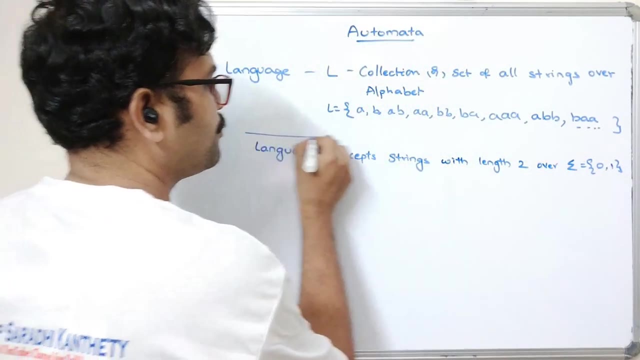 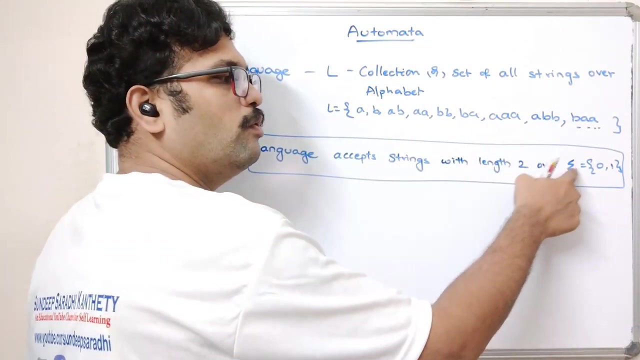 Sigma is equal to 2 over the alphabet 0 comma 1, so this is the question. okay, this is the question. so we need to have the language which accepts the strings with length. 2 over sigma is equal to 0, 1, so here the sigma is 0, 1 and we have to construct all the strings. 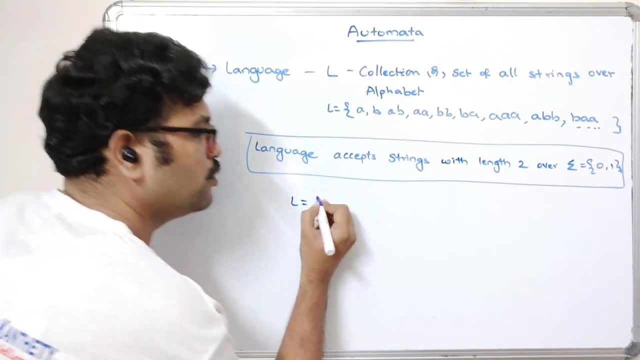 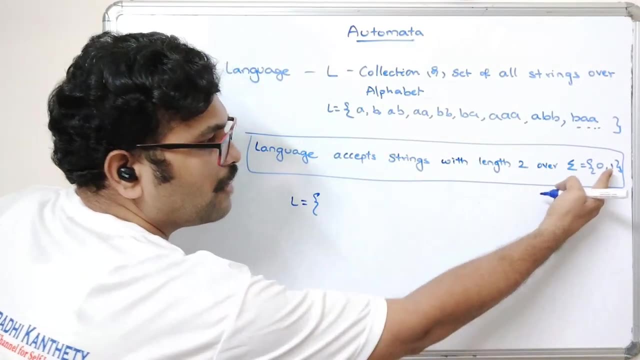 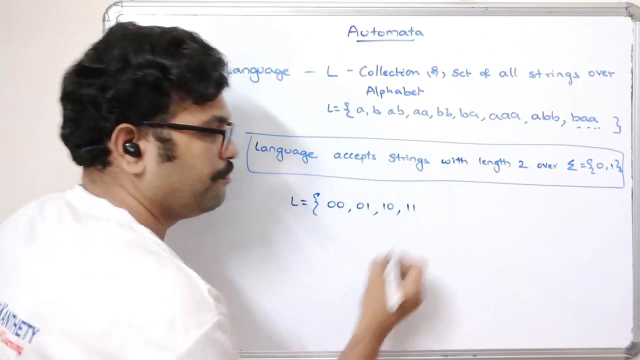 of this particular language, so language L is equal to, so it should have the strings with length 2.. Okay, So here you can see. the alphabets are 0- 1,, so 0- 0,, 0- 1,, 1- 0,, 1- 1,. okay, so this is the. 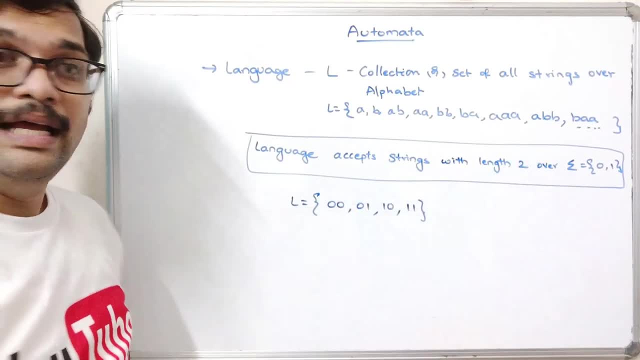 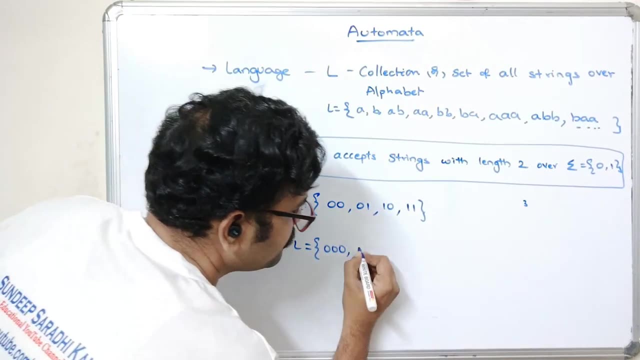 language of length 2, if we take length 3, so we will get so 0 0, 0,, 0, 0, 1, 0, 1, 0, 0, 1, 1, 0, 1, 1.. 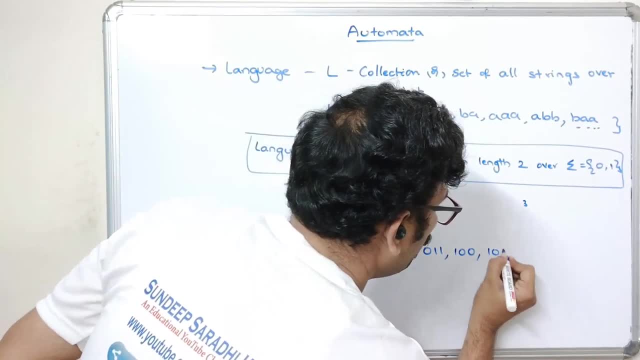 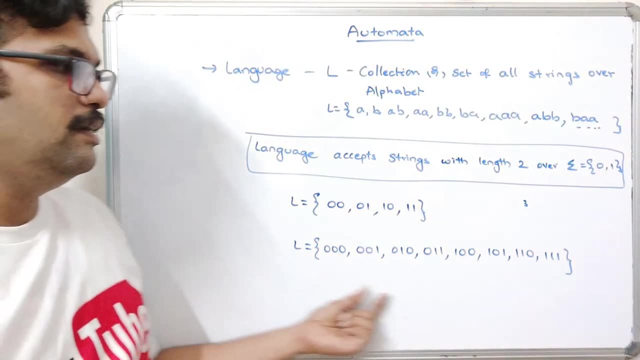 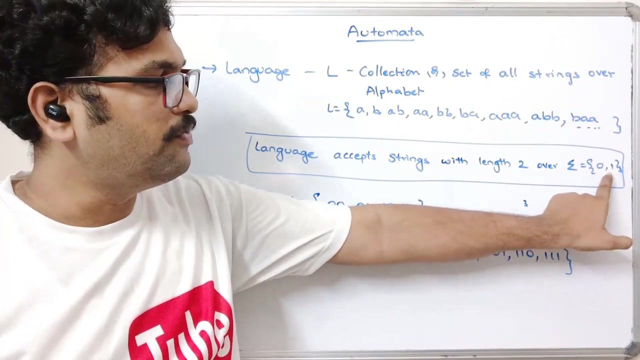 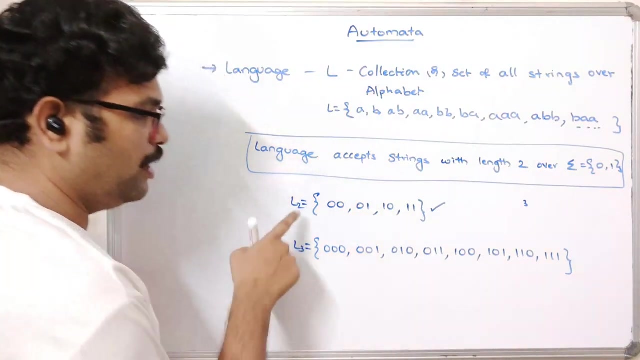 So these are the different languages. okay, these are the different strings that can be formed from this particular alphabet. so you can see whether L or I mean see. here you write L 2 and here you write L 3,. L 2 means length 2, length 3, so both are finite. 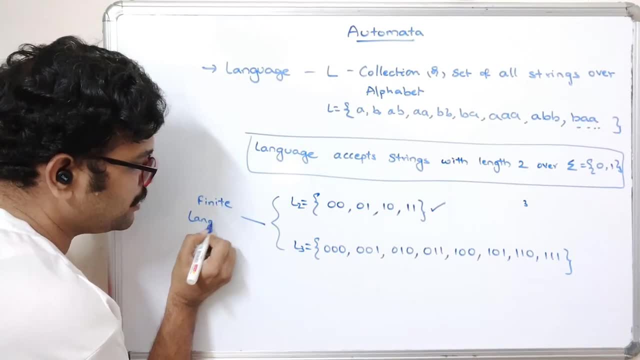 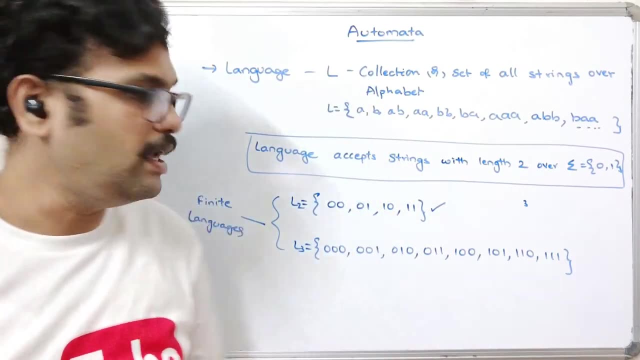 languages, Right, so we can't say that every language will be a finite. so that can be a finite or infinite. okay, Now we will see the strings with a length greater than or equal to 2, so if it is greater.